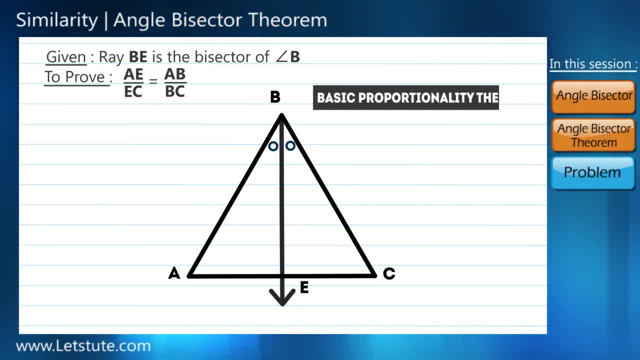 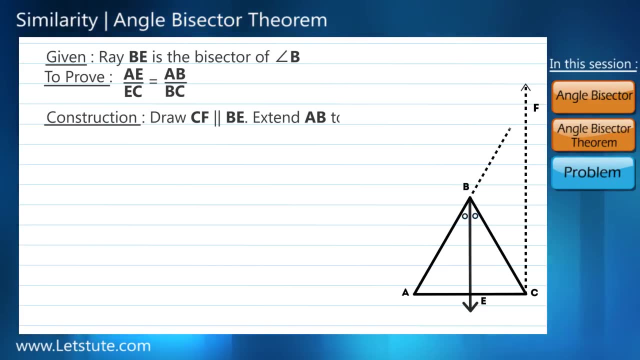 As mentioned earlier, we will be using the basic proportionality theorem itself to prove this. So let's do small constructions: that we draw ray CF parallel to ray BE and extend AB to intersect ray CF at point F. Now if you look at the bigger triangle formed here, that is triangle ACF. 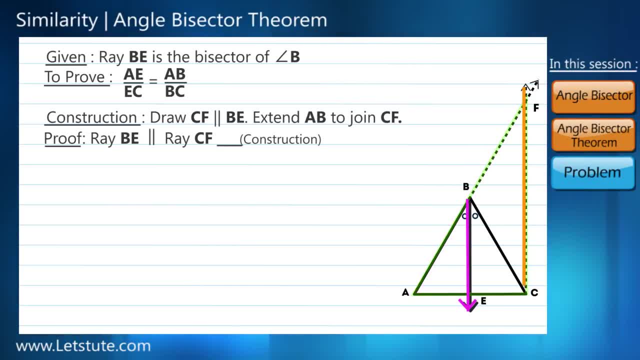 ray BE is parallel to ray BC. That means ray BC is parallel to ray BC. Now if you look at the bigger triangle formed here, that is triangle ACF, as per our construction, Can we write: AE upon EC is equal to AB upon BF. 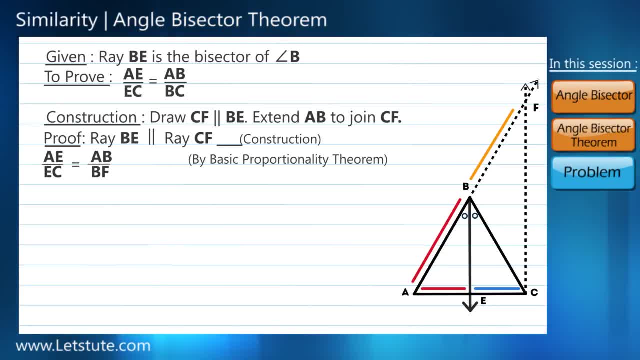 Yes, by basic proportionality theorem. Name this equation as equation number one. Now, if we carefully observe the two proof, part AE upon EC is equal to AB upon BC. We have the LHS, that is, the left hand side, same in both the cases. 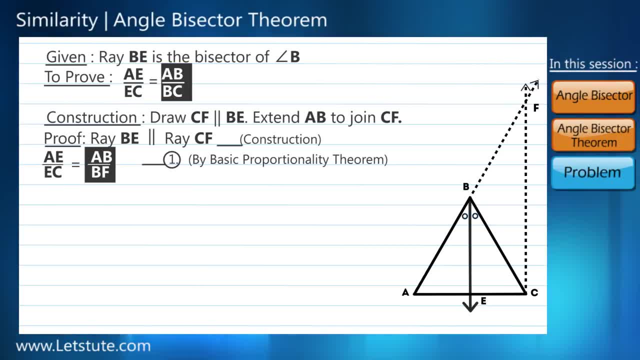 In the right hand side we have the LHS. that is the left hand side, same in both the cases. In the right hand side we have the LHS. that is the left hand side, same in both the cases In the right hand side. if we can somehow prove that length BF is equal to BC, 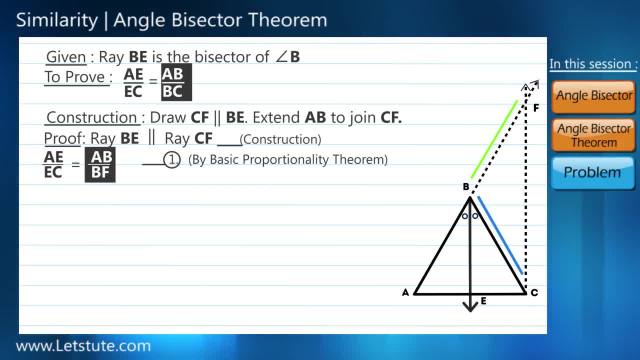 which are the sides of the smaller triangle formed, that is BCF. which are the sides of the smaller triangle formed, that is BCF. we are all sorted. Let's figure out how to do that Here. we know that ray BE is the angle bisector of angle ABC. 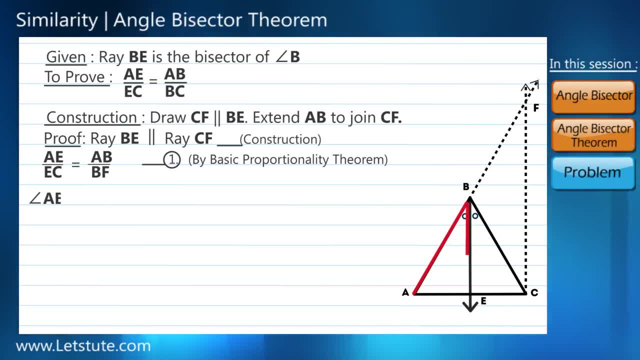 So we can write it as: angle ABE is congruent to angle EBC. So we can write it as angle ABE is congruent to angle EBC. Now let's consider the two parallel lines, BE and CF and AF as the transversal. 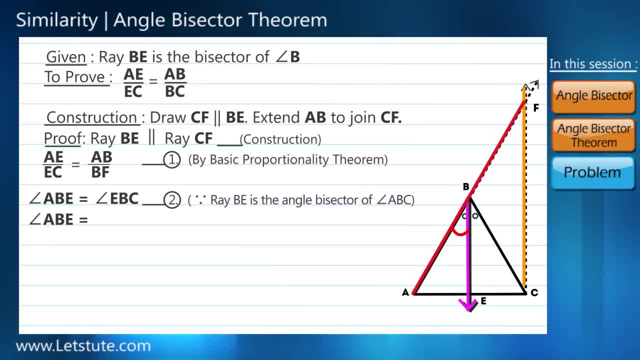 Now let's consider the two parallel lines BE and CF and AF as the transversal. We get angle ABE is equal to angle BFC as they are the corresponding angles. Now, considering the same two parallel lines, BE and CF, and BCF, as the transversal, 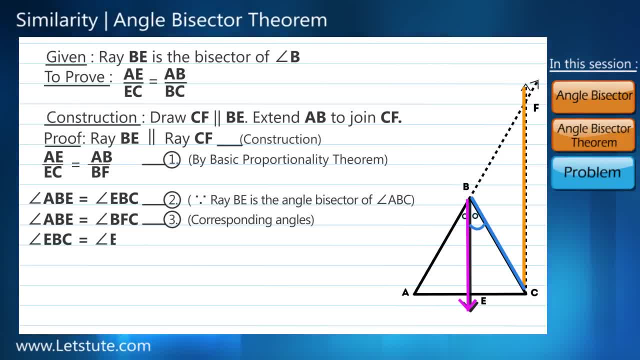 we get angle EBC equal to angle BCF. So now we get angle BF equal to angle BCF, as they are the opposite angles, making up the alternate angle as they form the alternate angles. Now, if you see the three equations 2, 3 and 4,, 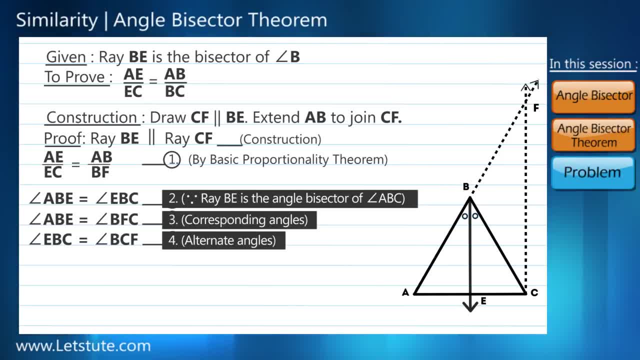 Now, if you see the three equations 2,, 3 and 4, can we say that angle BFC is congruent to angle BCF? Yes, and now BF will be congruent to BC, as they are the sides opposite to congruent angles. 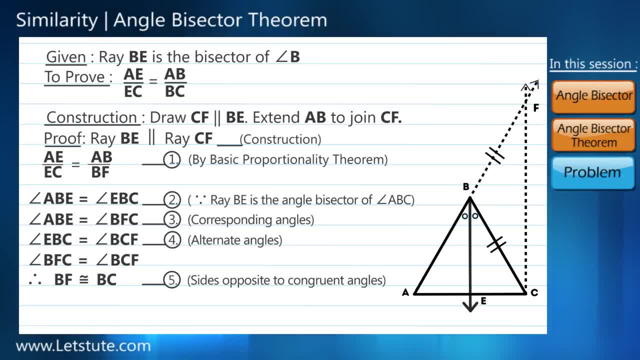 Here we have actually proved the sides congruent. Here we have actually proved the sides congruent. Now, from equation 1 and 5, we can write: AE upon EC is equal to AB upon BC. So here we finish the proof. and now we can rightly say that the angle bisector of a triangle 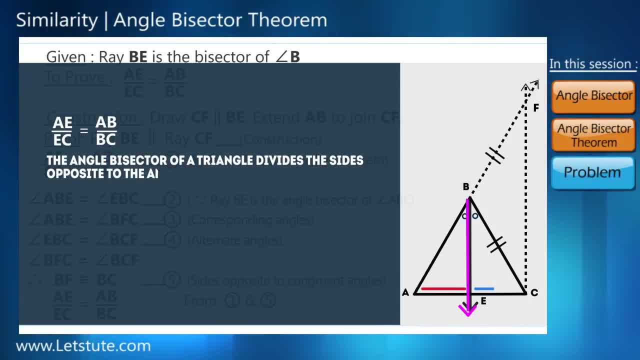 divides the side opposite to the angle in the ratio of the remaining sides. Now, if AE upon EC is in the ratio of 1 by 2, then AB upon BC will also be in the same ratio. Here I am not talking about the length, but the ratio of the lengths. 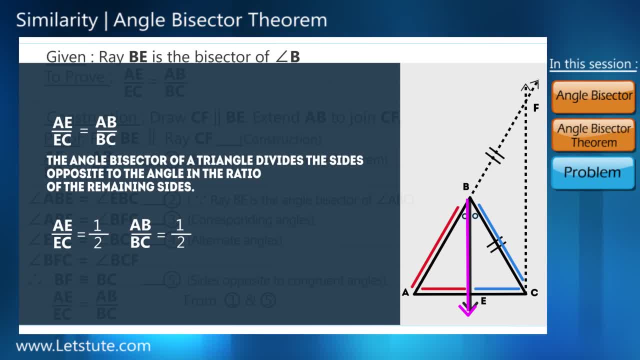 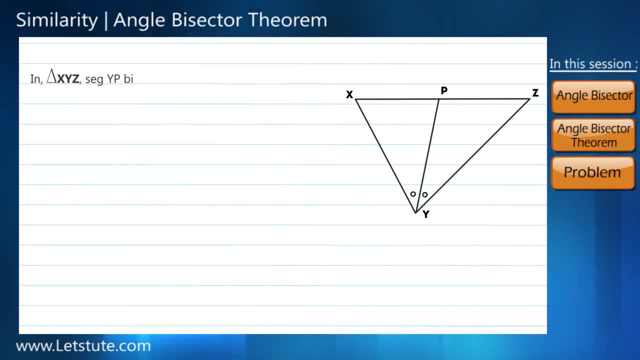 Hope the concept is clear. now Let's move a step further and solve a problem related to the same. In triangle XYZ, segment YP bisects angle XYZ. If length XY is equal to the length of the triangle, then the angle bisector of the triangle is equal to the angle of the triangle. 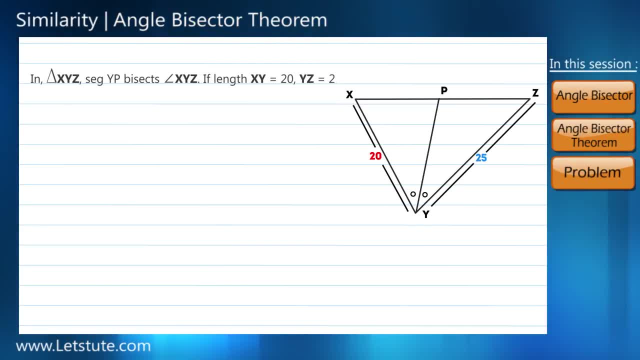 If length YZ is equal to 20, YZ is equal to 25 and PZ is equal to 15, then find XP Very simple and straightforward question. We just have to use the same concept that we have just studied In the figure XYZ. segment YP bisects angle Y. 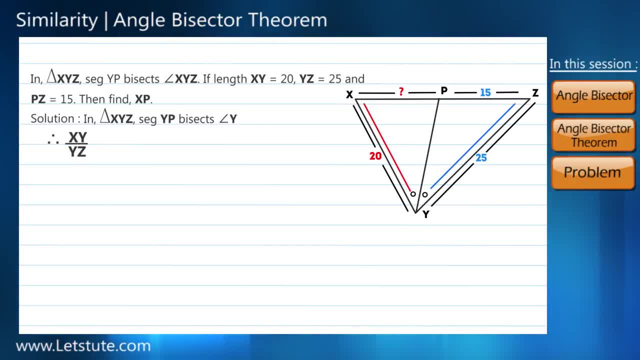 Therefore, XY upon YZ is equal to XP upon PZ. By the property of angle bisector, Let's put the values: 20 upon 25 is equal to XP upon 15.. Solve it further Now we get XP as 12.. 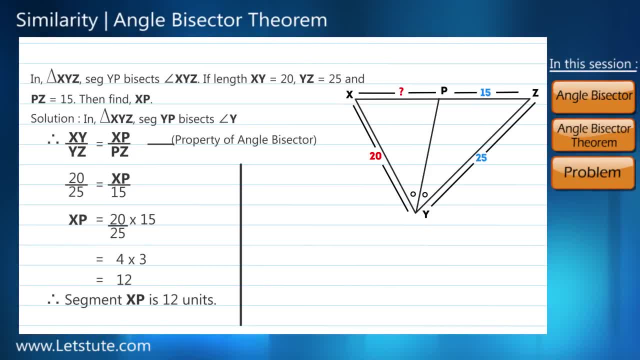 12 units. On getting the lengths, you may even check their ratios. Yes, it is coming 4 by 5. So we are correct. With this we end our session. Hope you are thorough with the property of angle bisector.